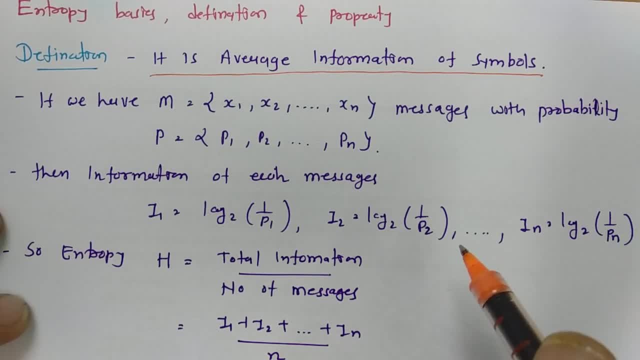 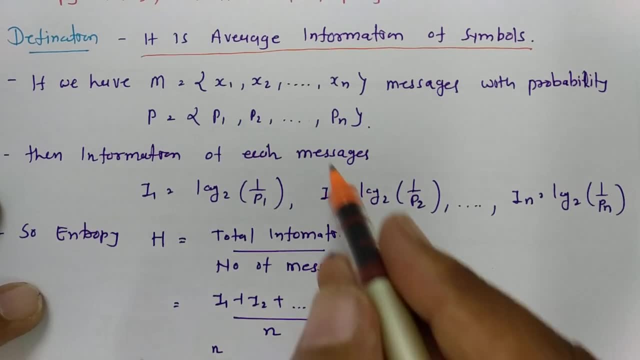 log of base 2 of 1 by p1.. So this is what the basic definition of it is. So let us begin it. Log of 1 by pn base 2.. So entropy is what exactly? Total information divided by number of messages. So here n number of messages are there. So total information is i1 plus i2 up to 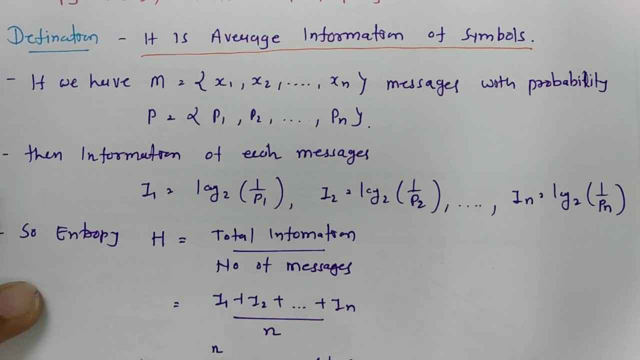 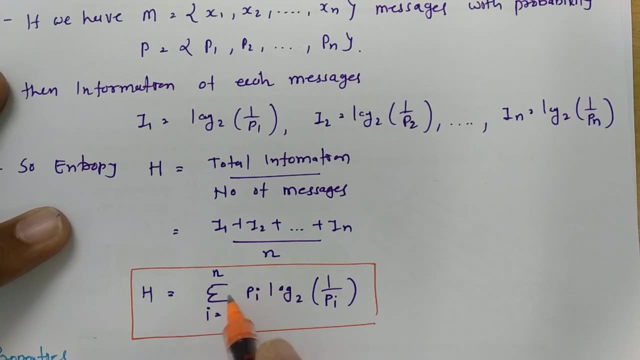 i and divided by total messages, that is n, And if you solve that you'll be finding entropy formula will be this And that is summation of: i varies from 1 to n pi log of 1 by pi base 2.. So this is what very important formula that one should know And its unit. 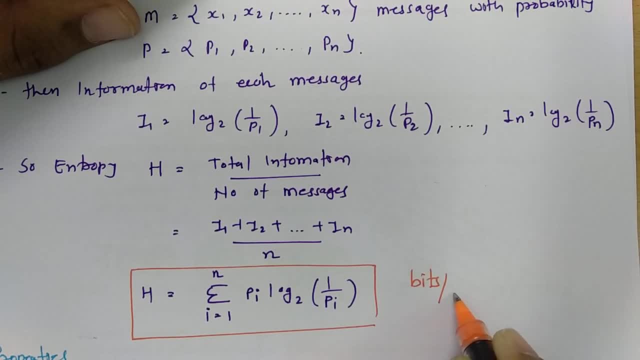 that is bits per symbol or message. So its unit is bits per symbol. So that is what the basic formula that we should remember to solve examples. So entropy basic formula is summation varies from 1 to n pi log of 1 by pi base 2.. So this is what very important formula that one should know. 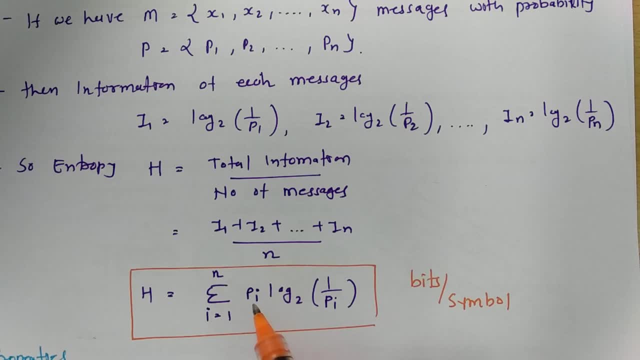 And its unit is 2.. For information calculation you don't have pi multiplied here. For entropy you will have to multiply pi over here. So this is what the basic difference in between information and entropy. Information unit is bits and entropy unit is bits per symbol. 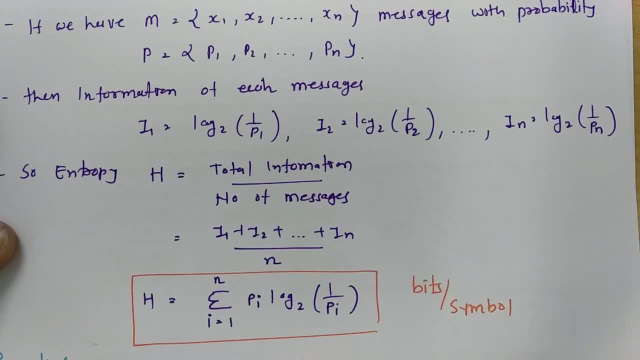 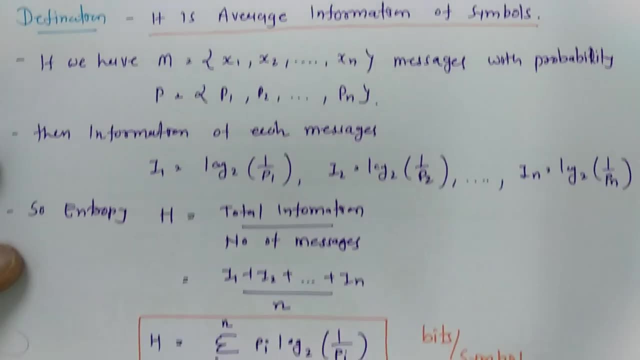 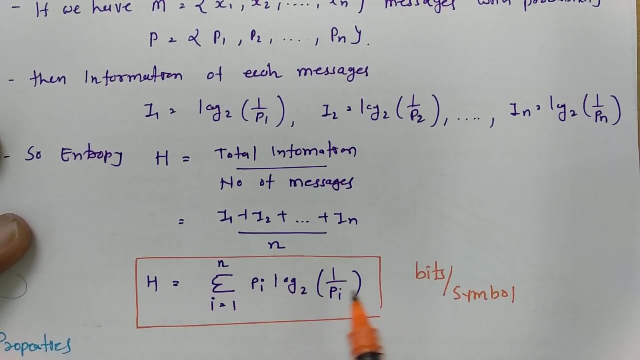 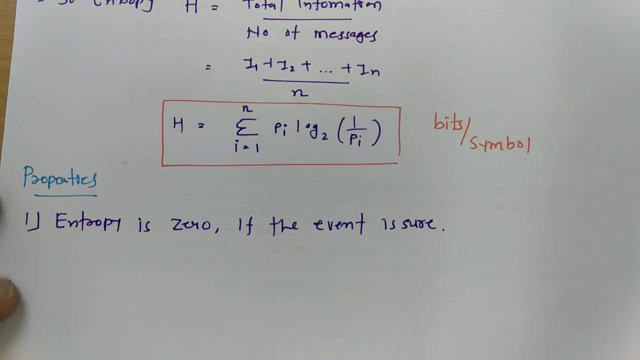 So this is how units are different. So again see the definition is: it is average information of symbols And basic formula is: it is summation pi log of 1 by pi base 2.. So this is how we can calculate entropy. Now let us see what are the basic properties which is there with 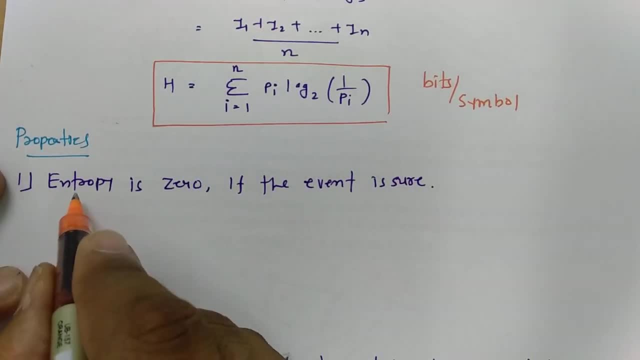 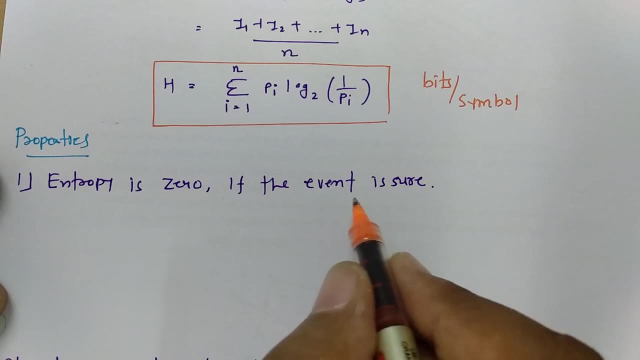 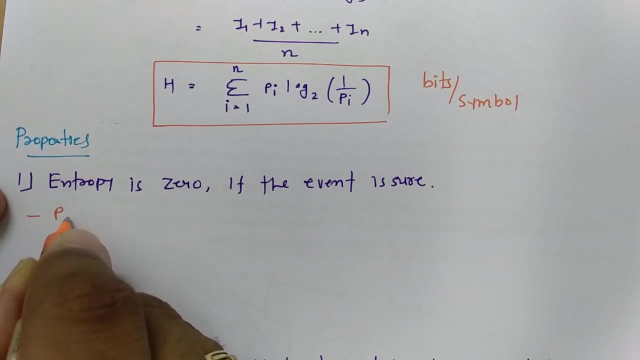 entropy. So see first property, that is, if entropy is 0, if event is sure. So this is what first property. So let us prove it. So if event is sure, what it means? Probability can be 0 or probability can be 1.. So if probability 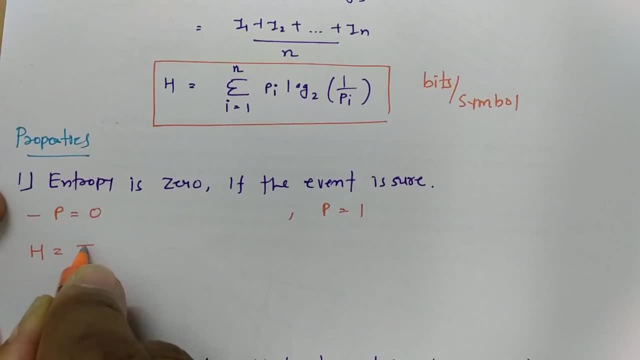 is 0, then entropy basic formula is summation: k varies from 1 to m pk log of 1 by pk right. So if probability is 0, so anything multiplied with 0 will result into 0. So we can say: 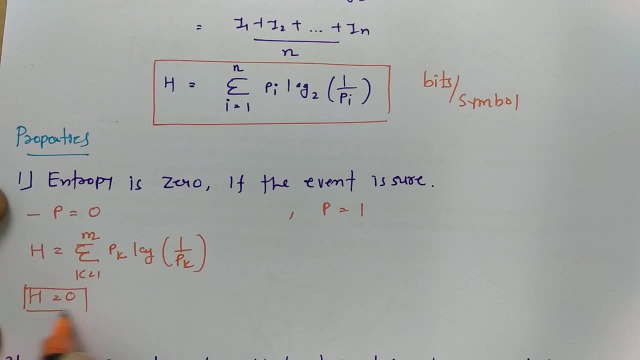 over here. entropy is 0.. Now let us check it for second case. So, as we know, the basic formula summation k varies from 1 to m. pk. log of base 2, that we need to remember- 1 by pk. 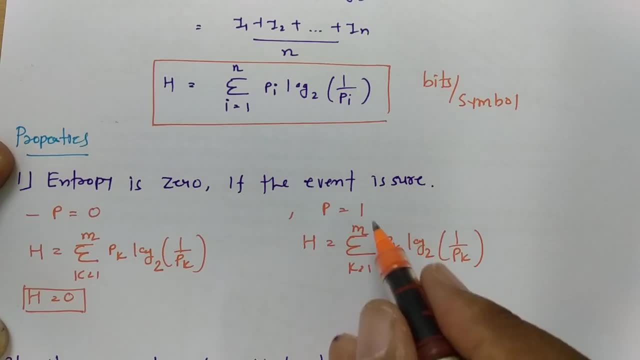 So if you place probability is equals to 1 here, then you will be finding it is 1 log of 1 divided by 1 base 2 and log 1 that is 0. So this case, even results into h, is equals. 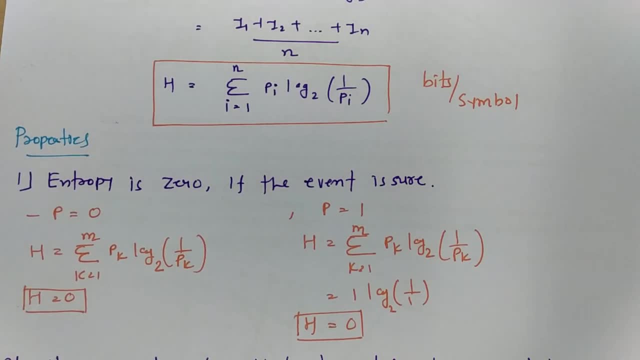 to 0.. So, ultimately, if event is sure, like if we know what is the probability of k being 1, then we can say: over here, entropy is 0. So what is that event which is happening? In that case one can say there is no information. 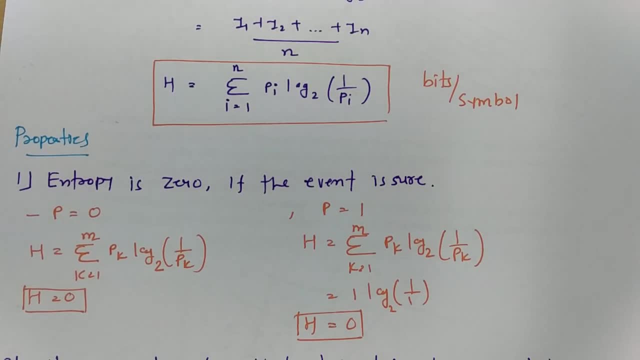 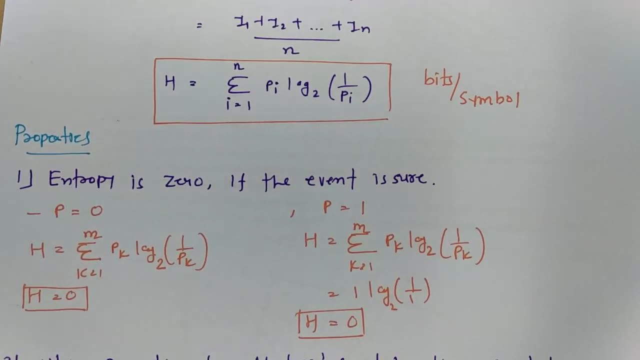 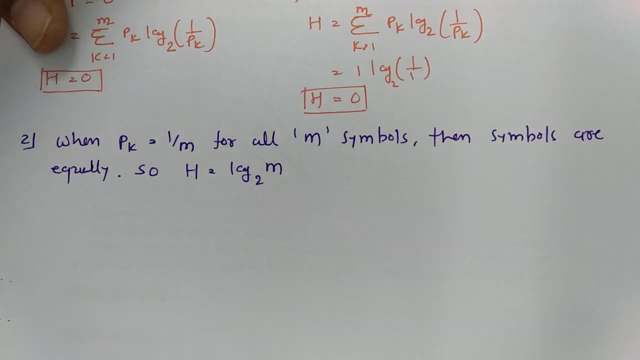 The reason is that information is already known, So entropy regarding that will be 0, and that is what we can prove even by this basic calculation. Now let us have one more property of entropy. See in this property when probability is 1 by m for all m symbols. 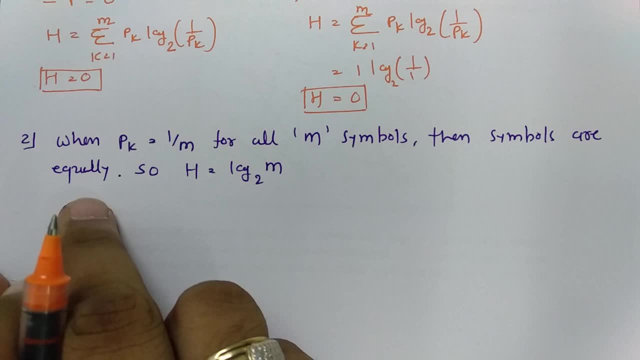 then the symbols are 1 by m, So this is the probability of k. So if probability is 1 by m, then the symbols are equally. then symbols are equally so that h is equals to equally probable, so that h is equals to log of m, base 2.. So this is what we are delivered to prove. 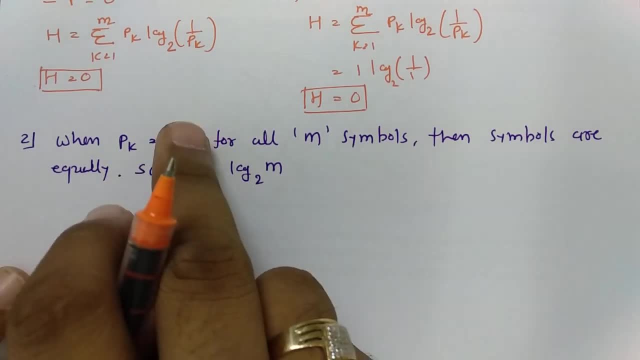 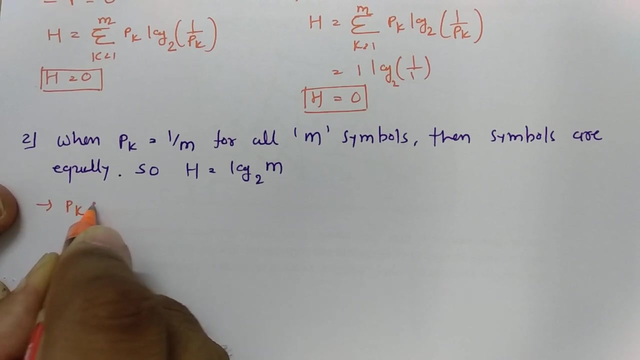 about. So here, probability of all symbol is 1 by m. So we need to identify what is that entropy and that should be this. So let us try to derive it. So let us try to derive it. So, as we know, probability that is given for all symbols, that is 1 by m. 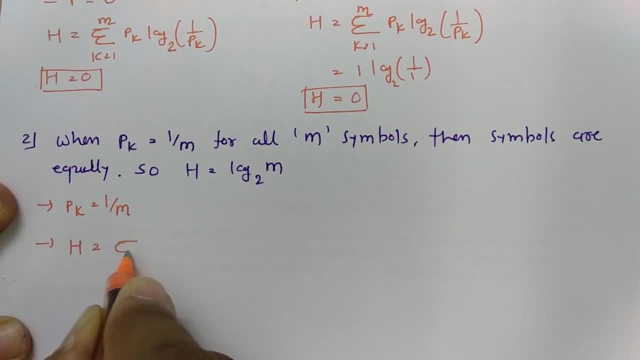 So entropy h is equals to. as we know, the basic formula k varies from 1 to m pk, log of base 2 to 1 by pk. So let us place: pk is equals to 1 by m in this. So this is the. 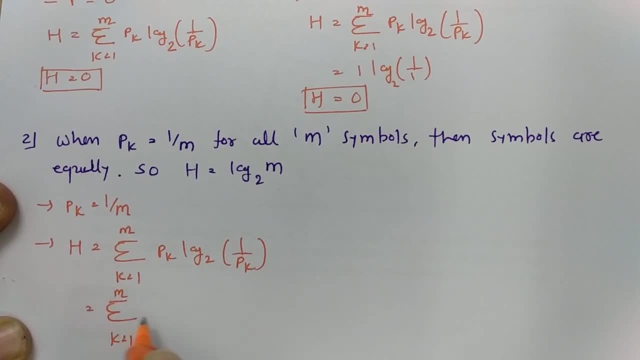 probability of k. So this will be summation. k varies from 1 to m, 1 by m into log of base 2 and 1 by m. 1 by pk means 1 divided by 1 by m, So that m will come in numerator Now. 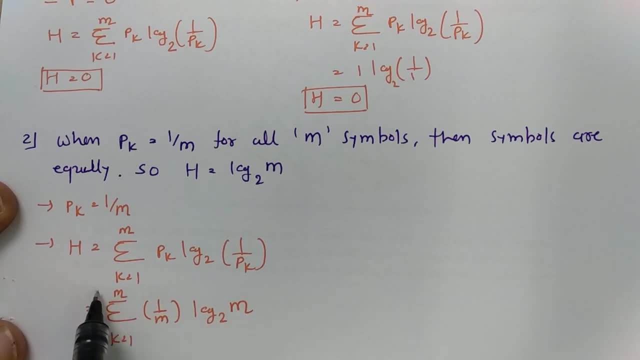 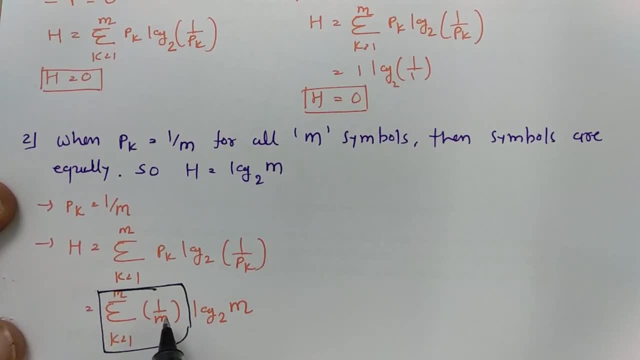 It is actually 1.. So if you add 1 by m m times, so that will result into 1.. So this summation is resulting into 1.. It means it means this: h, that is equals to log of m base 2.. So for 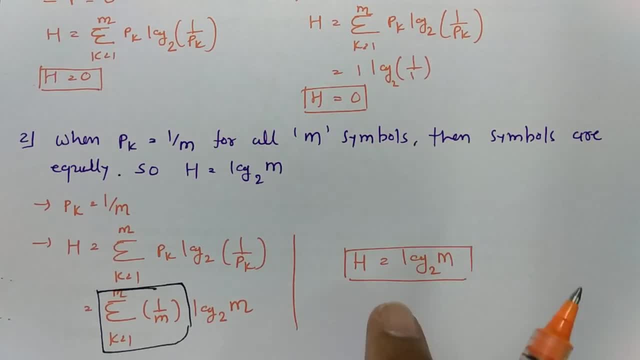